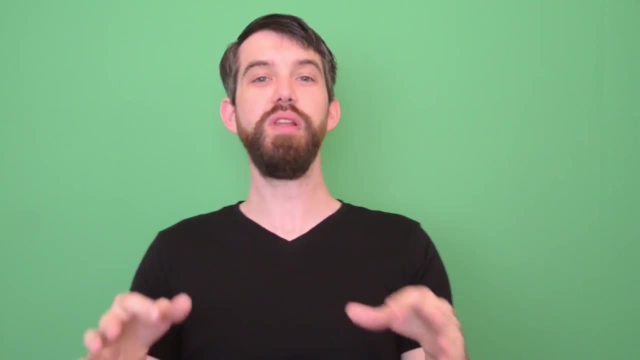 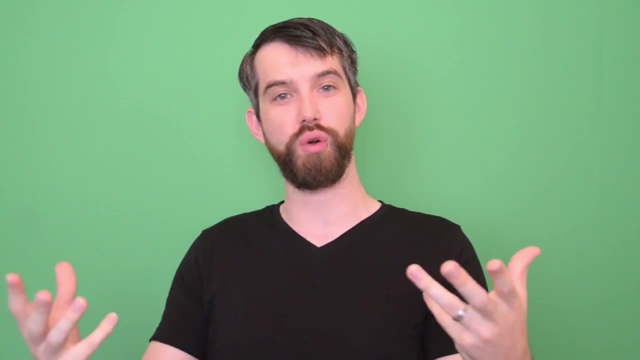 Welcome everybody. In this video I want to give you a little bit of a sense of what the rest of our semester is going to look like. I'm going to talk about some discrete math. I'm going to talk about the structure of our course and a little 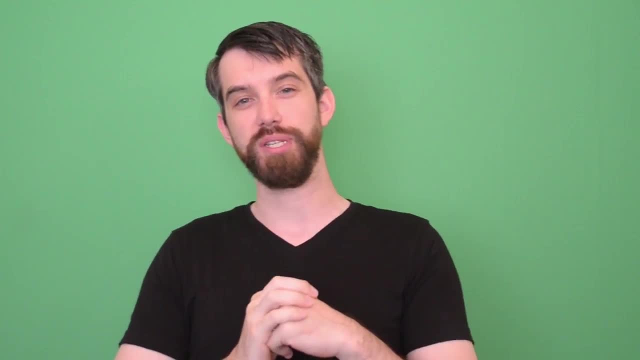 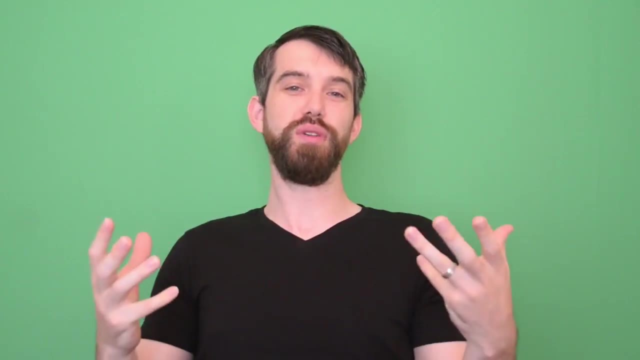 bit about how to succeed in the context of this online course. So, first up, what's discrete math? anyways, I like to think of it as a wonderful introduction into mathematical thinking. Indeed, we're going to learn how to think logically, to think. 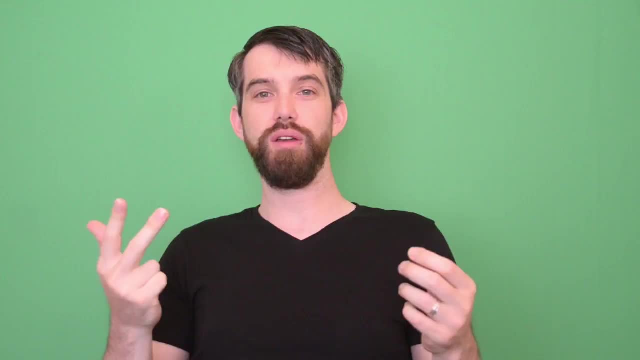 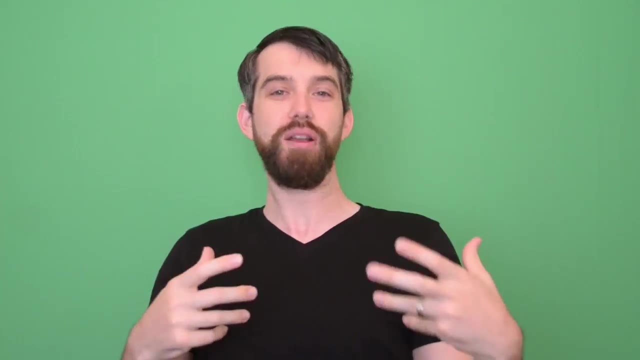 rigorously to think symbolically and also to think creatively, which might seem like his intention with those other things. but I don't believe that's the case And indeed in my background I actually started university in computer science and then I took a discrete math course and I kind of fell in love with 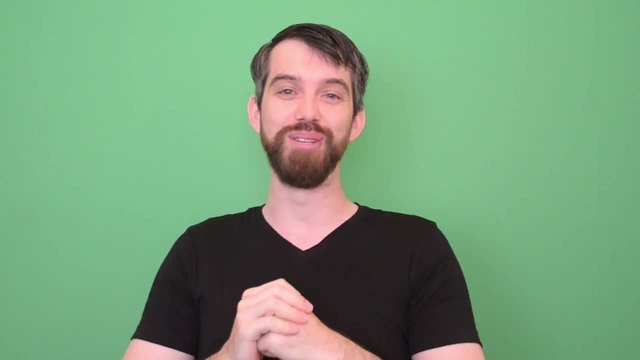 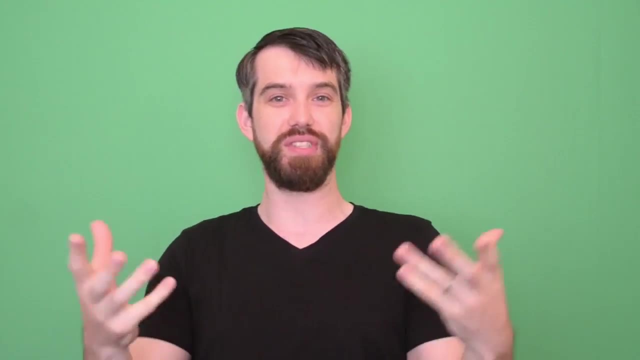 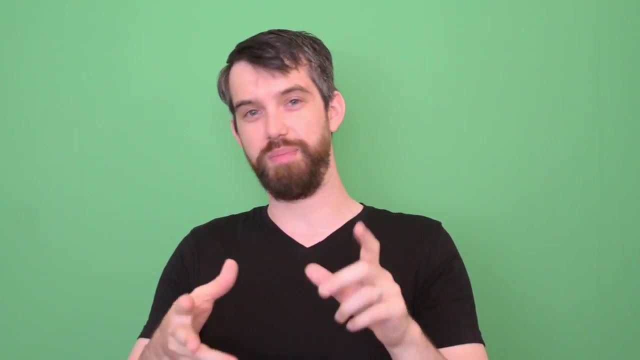 mathematics and mathematical thinking. and well, here I am now as a mathematics professor. I was taken to the dark side, But discrete mathematics takes this sort of set of skills and applies it to a kind of math problem. that's particularly useful for people in computer science and people. 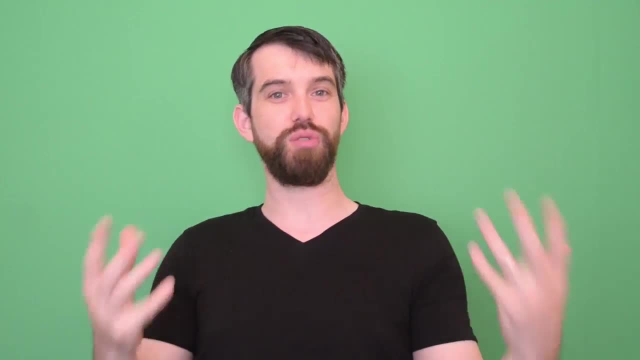 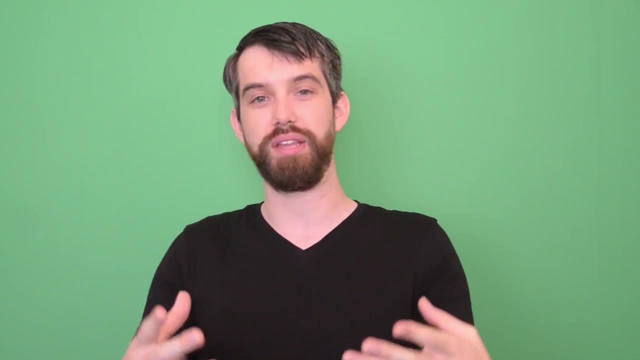 in information technology And the idea of discrete mathematics is in contrast to the kind of sort of continuous mathematics that some of you might have seen in high school or if you ever took a pre-calculus or a calculus class where, for instance, if you consider the function x squared that when you think about this, 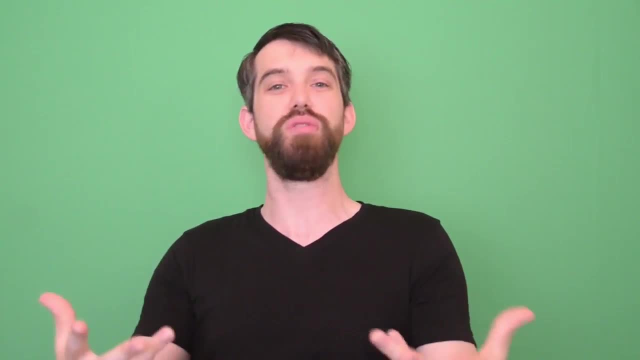 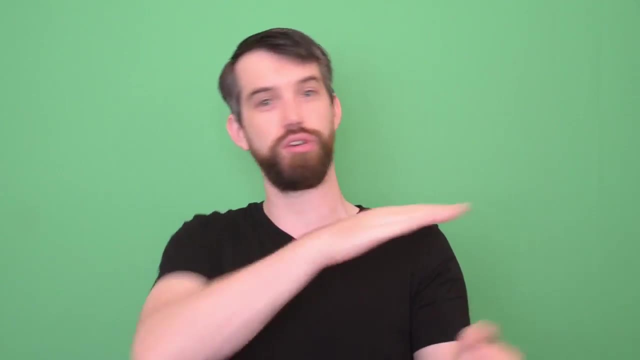 in the past we've often thought of it. where you're allowed any real number, x could be the input, not just one and two, but a half and a third and a quarter, and pi and root two and all sorts of things, a sort of continuous number line of. 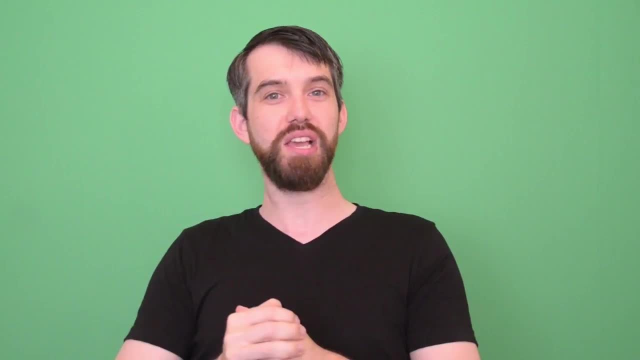 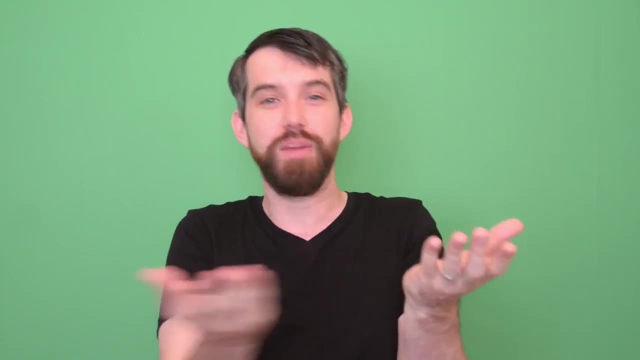 possible inputs. In discrete mathematics we try to think of the basic entities that we're going to talk about as sort of separate. things like one and two are separate and they're not connected by the whole set of numbers in between them. We might be 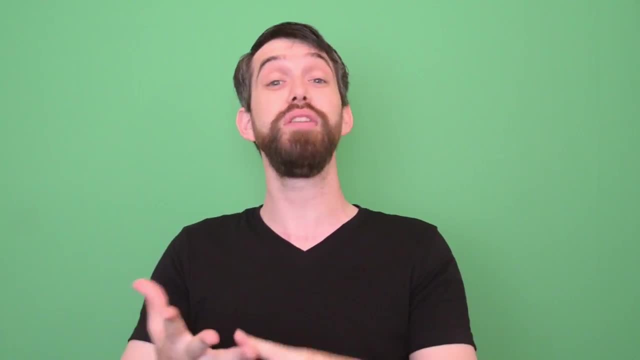 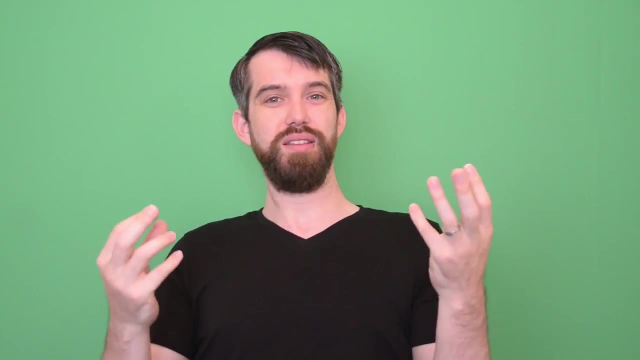 interested, for instance, only in the integers, numbers like 1,, 2,, 3,, 4, but not necessarily all real numbers, the numbers in between it. Now, the reason why discrete mathematics is so important is because it's a very important part of the 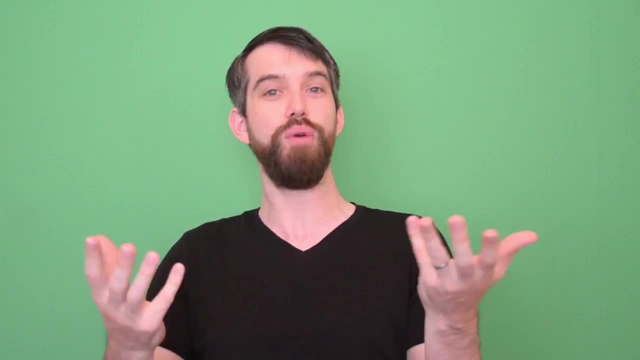 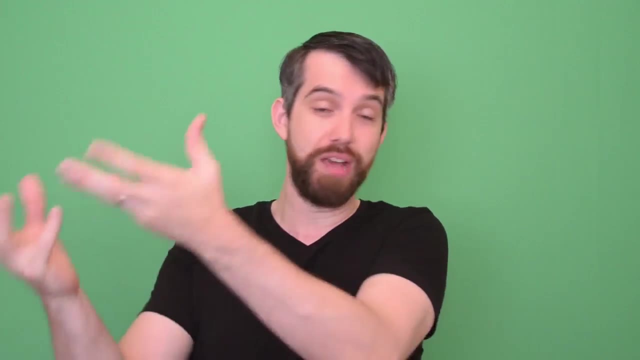 computer science and information technology is that's how a lot of information technology stuff works. For example, if you have a database, you have just discrete entries and they might have a bunch of different properties, but you usually don't have sort of a notion of one-third of the way between two. 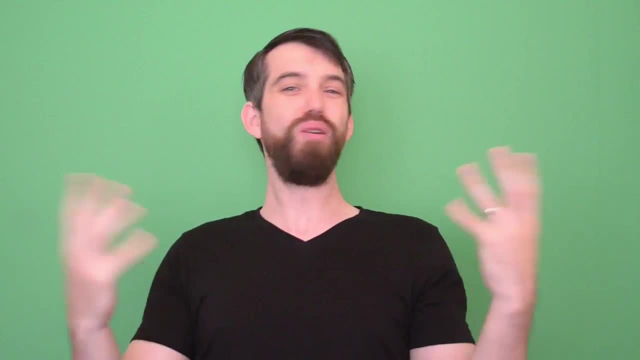 different entries in a database. And so in this course we're going to do all sorts of different things. We're going to do probability, we're going to be doing counting, we're going to try to get to a little bit of graph theory. we're just going to do some. 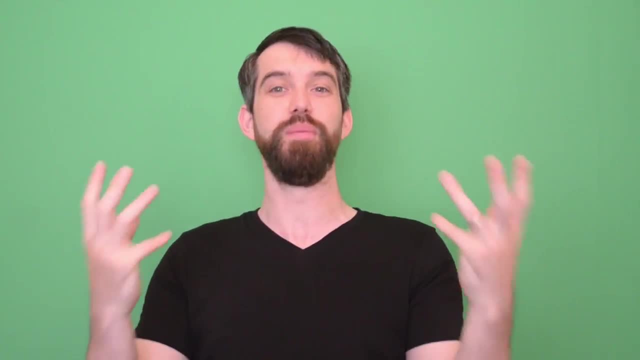 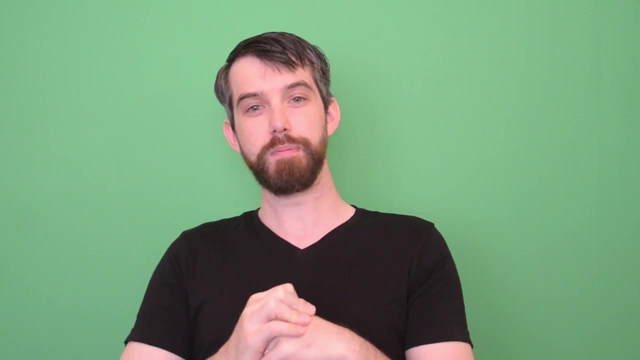 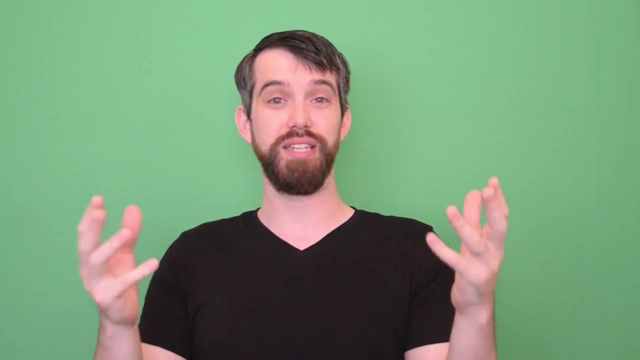 basic logic stuff at the beginning of the course so that we feel empowered with our own logic And all these different things that are going to have a lot of application throughout computer science and information technology. Now, this is an online course and online courses can be kind of challenging for students because you don't have that constant, continuous 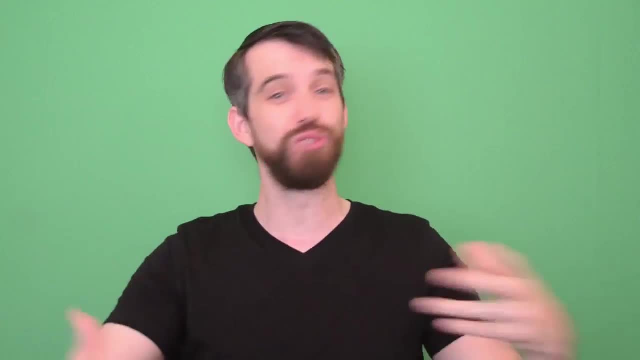 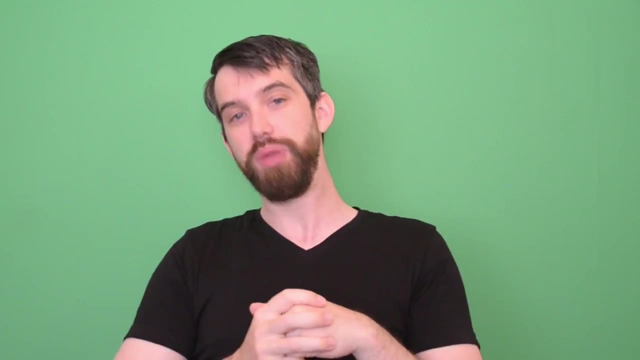 structure of you've got to go to class and you have this sort of social pressure to show up and do whatever the teacher is doing In an online course. a lot more of that momentum is going to come from you, So I'm going to give you just a little bit of the scaffolding. 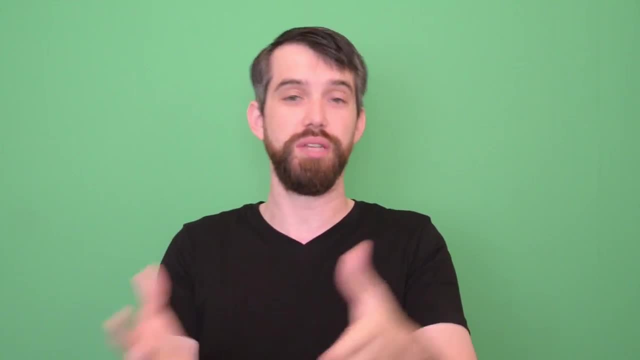 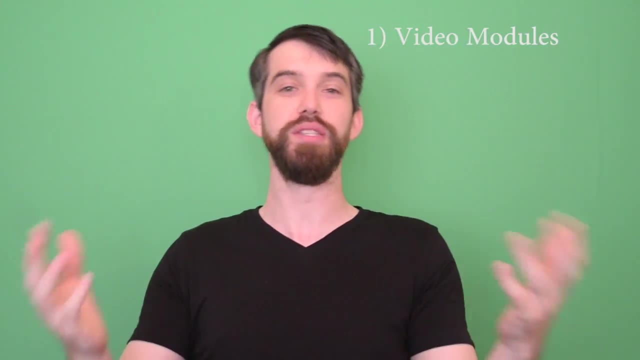 that I'm going to use in this course That I'm hoping that you can use to master your learning of discrete mathematics. So the first part- and you've probably already seen one of these- is the online video and quiz modules, And you should think of this as sort of the foundational knowledge. This 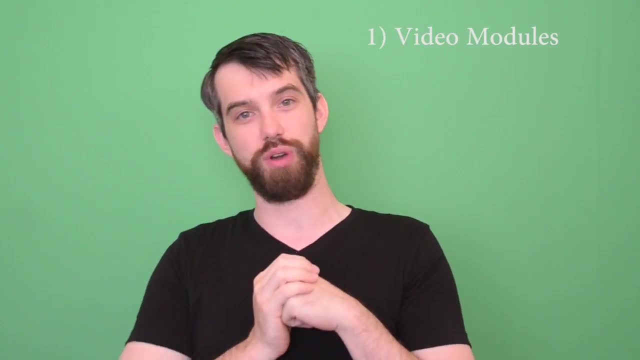 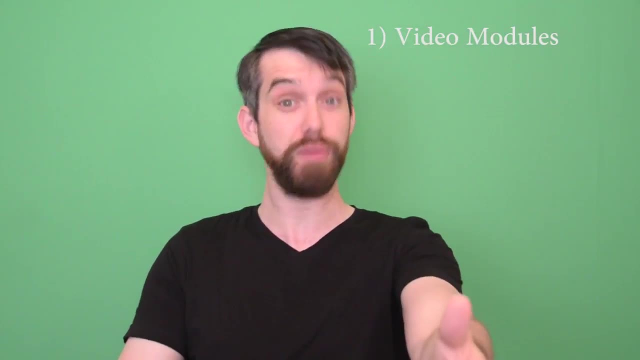 is us establishing the basic idea of whatever section we're going to be doing, but it is absolutely not in learning the material to mastery. That is something for you to do. You have to take the sort of initial video module as sort of the springboard to become. 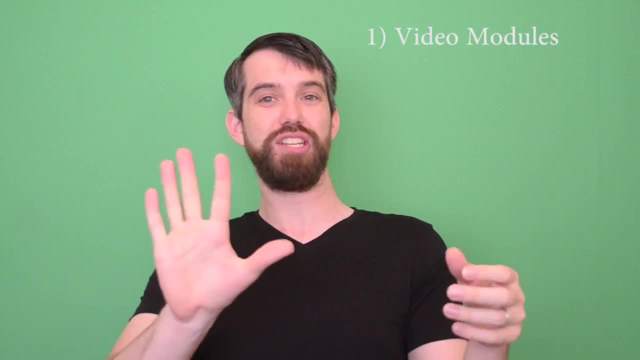 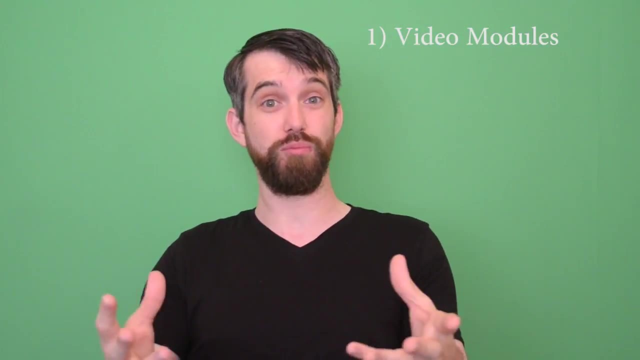 a master in the subject, And so the way I sort of structure this is really actually five different components. So we've got sort of the video modules first, But then I think it's a good idea to go and read the relevant portion of the textbook, But not just read. 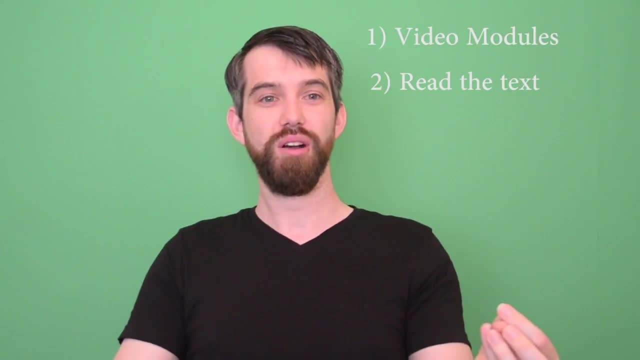 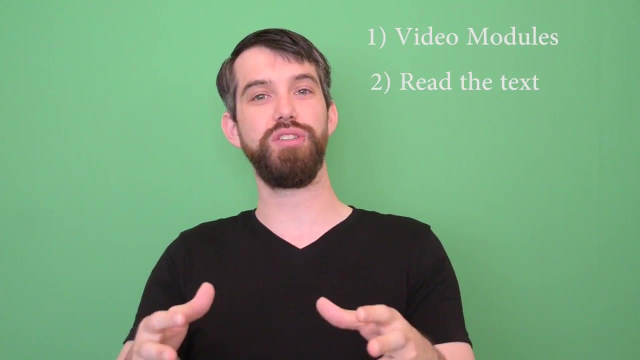 it like skimming it, Read it, like really analyzing it. Like what and why are they saying these things? Do you have any questions? Where is this going in the future? How do you connect this to prior content and to other content that you know? What's the main point of this? 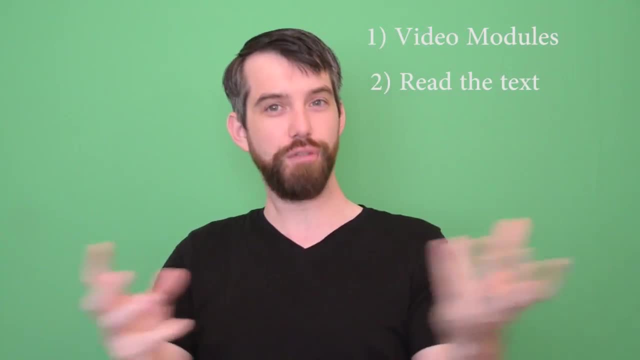 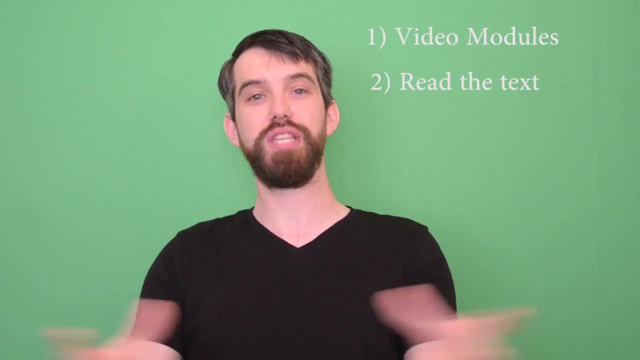 section. Are they all valid? That's the kind of questions you should be thinking as you sort of read over this textbook. So you sort of have this introduction from me in the video lectures And then you have to sort of do the deep dive in yourself through this section of the textbook. 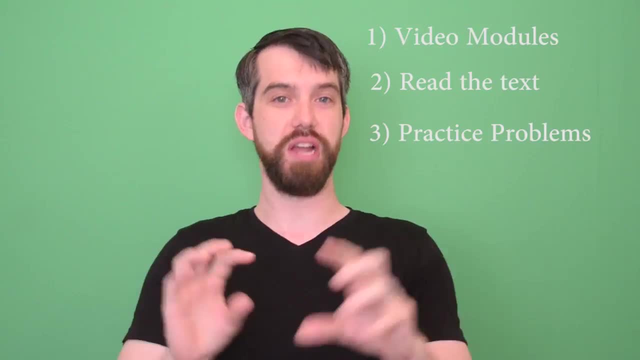 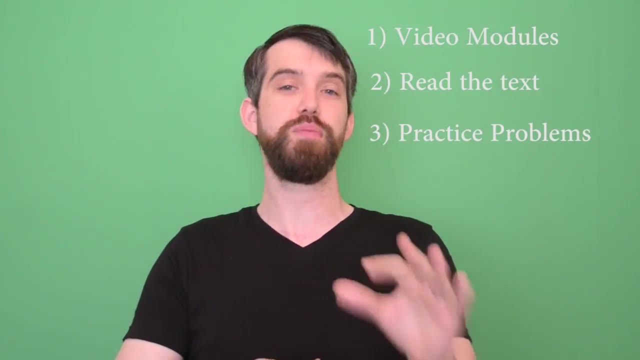 And that's on you, And then afterwards I'm going to always create a bunch of practice problems so you have some chance to practice, some problems and solutions will be posted. But I encourage you to try the problems on your own genuinely, as if it was a test. But